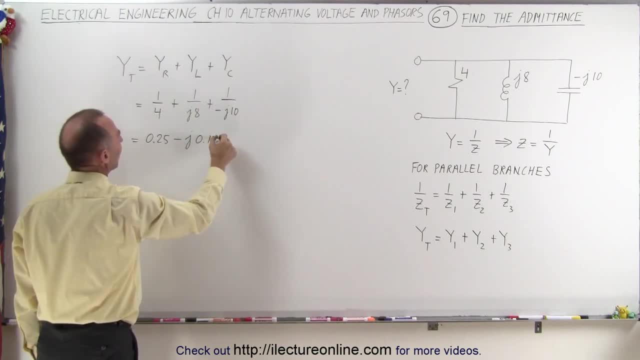 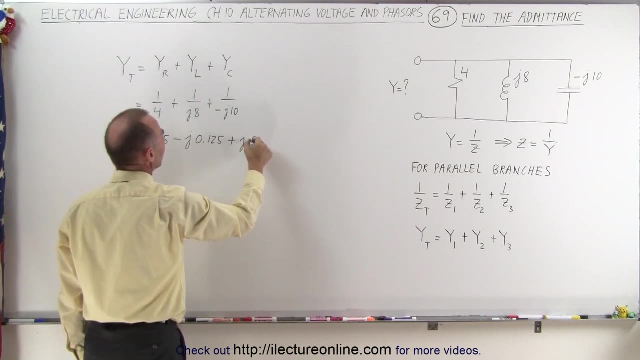 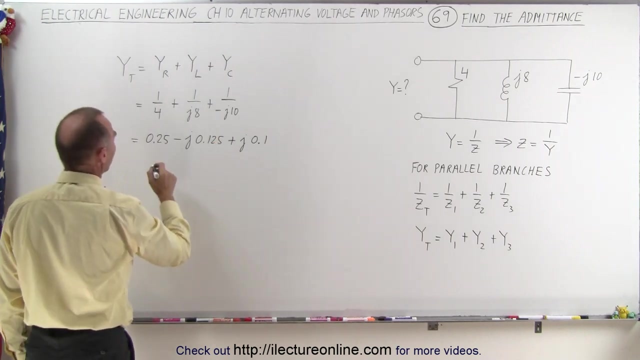 times 1 over J, which is 0.125.. And then here, when you bring the J to the numerator, it's minus times a minus that becomes plus J times 0.1.. So now this is the total admittance of the circuit. We can combine the two imaginary parts, So this is equal to 0.25, and that's bigger than that. so that would be minus J times 0.025. 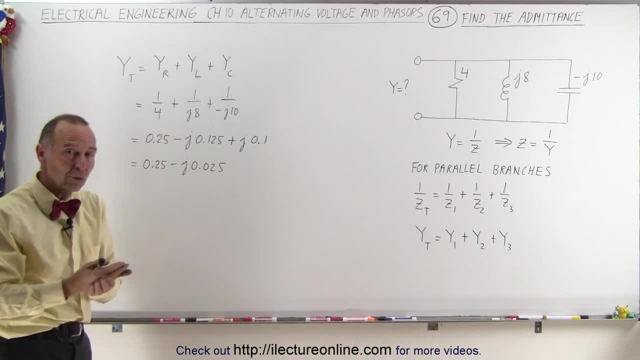 And then, if you want to write that into its magnitude and phase angle format, we can do the following. We can say: well, that's equal to 0.25. squared plus 0.025. squared is equal to that. divided by that, that's equal to: this is equal to 0.251, with a phase angle of that would be 1 tenth, so 0.1,. take the inverse tangent of that would be 5.71 degrees. a negative, negative, 5.1.. 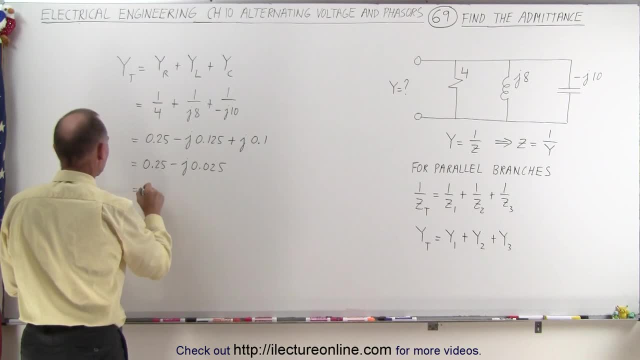 And then, if you want to write that into its magnitude and phase angle format, we can do the following. We can say: well, that's equal to 0.25. squared plus 0.025. squared is equal to that. divided by that, that's equal to: this is equal to 0.251, with a phase angle of that would be 1 tenth, so 0.1,. take the inverse tangent of that would be 5.71 degrees. a negative, negative, 5.1.. 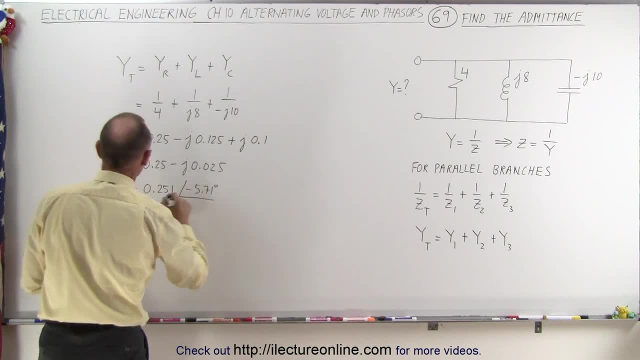 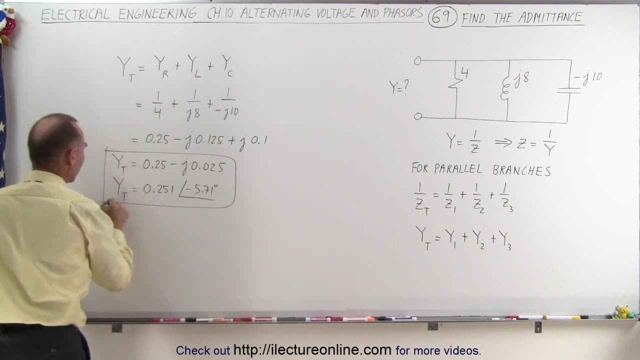 So that's equal to the admittance total, whichever format you want to put that in. So you can see that it's quite easy to find admittance for a parallel circuit. Now can we convert that into an impedance? And the answer is certainly. 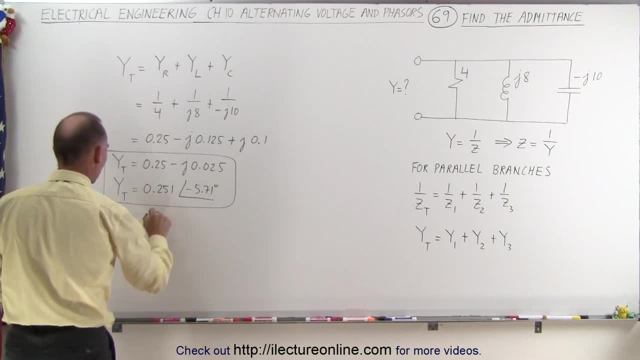 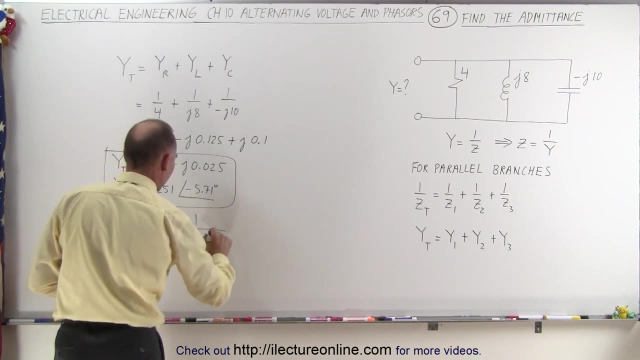 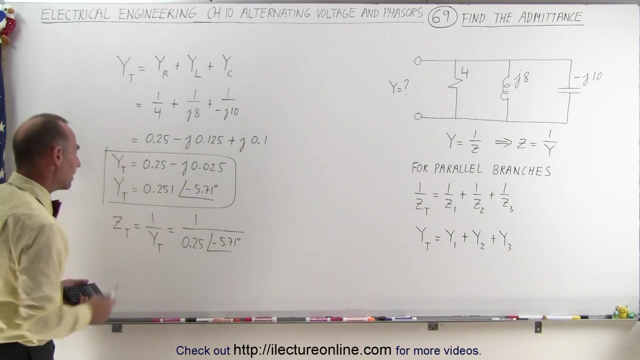 So the total impedance is equal to 1 over the admittance, which is equal to 1 over 0. 0.25 minus 5.71 degrees. so how do you take the inverse of that? well, first of all, this can be written as 1 to the 0 angle, because that's simply a number. so 1 divided by 0.25, that's equal to 4. 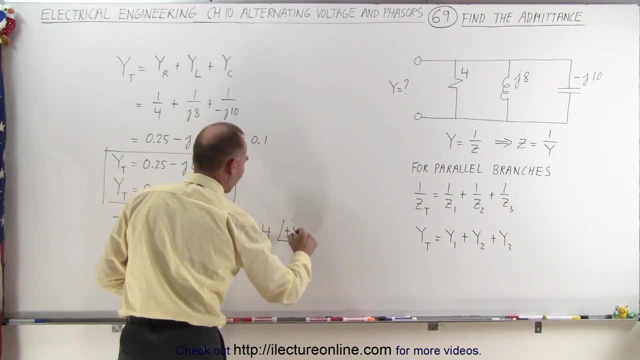 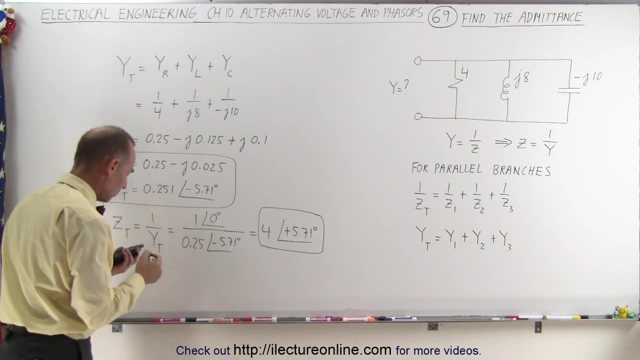 and then the angle becomes a positive 5.71 degree, and so that would be the impedance of the circuit, while this would be the admittance of the circuit. so it's quite easily. it's quite easily done by first finding the admittance and then reconverting back to the impedance. that's how we do that now.